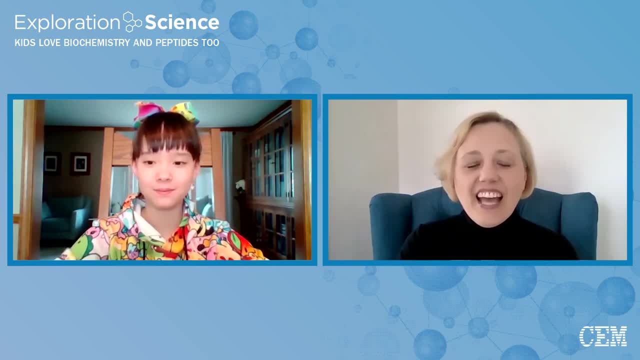 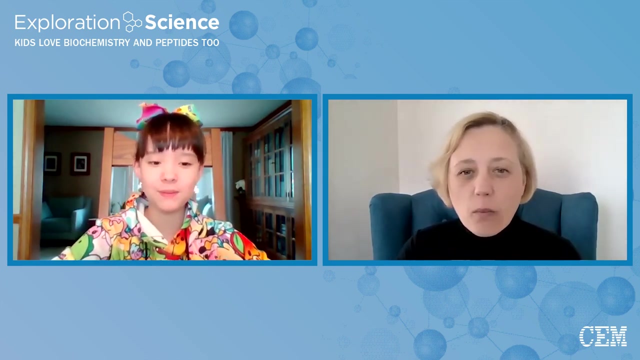 I live in Ohio, Ohio, Okay, excellent. I met some of your colleagues this morning in North Carolina and before that in Australia, So that was pretty fun. What grade are you in? I'm homeschools, but if I did go to school I'd be in fifth grade. But as you see, 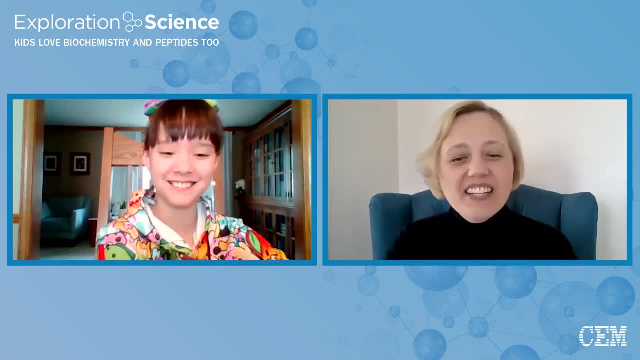 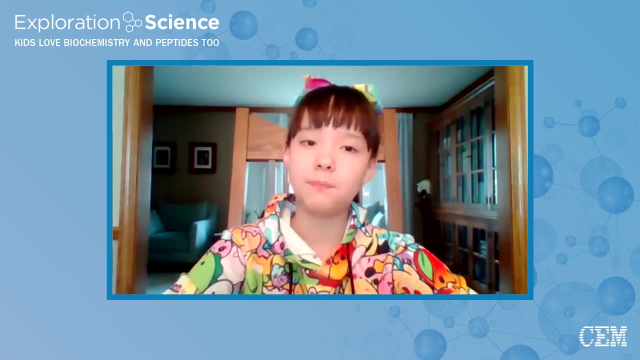 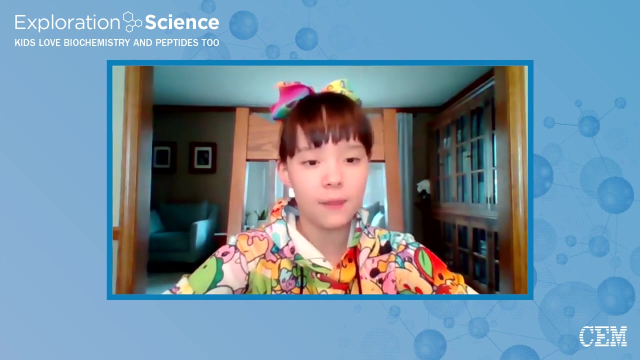 I don't just do fifth grade work. Yeah, absolutely Yeah. Tell me, how long have you been taking Dr Freed's class? Um, I think I started in the biochemistry beta class in like March of last year And then I switched to the alpha class because I had a schedule conflict. But I really 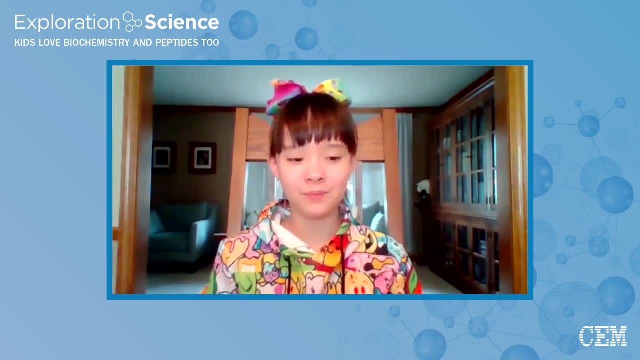 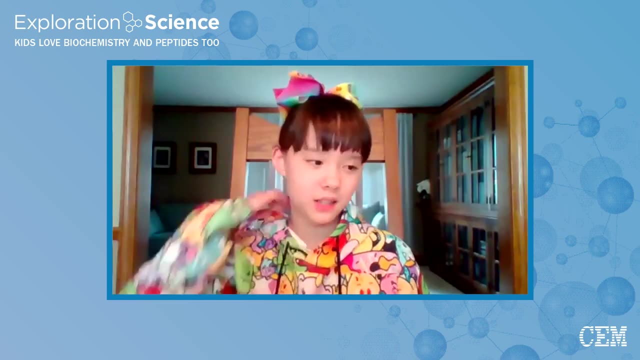 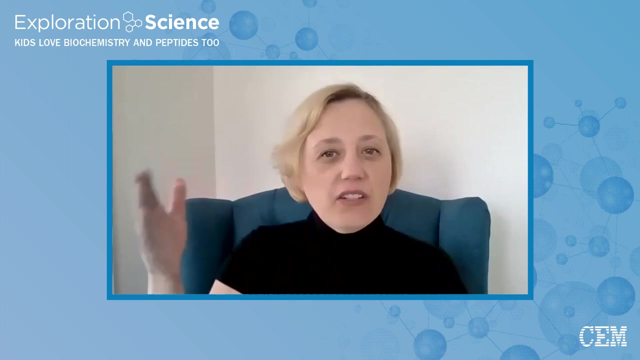 like the alpha class because, um, I don't know, I just do. What's the difference between the beta and the alpha class? Beta was the second group that he ever taught and alpha is the first group. So, yeah, So they were just a little further along in the curriculum. 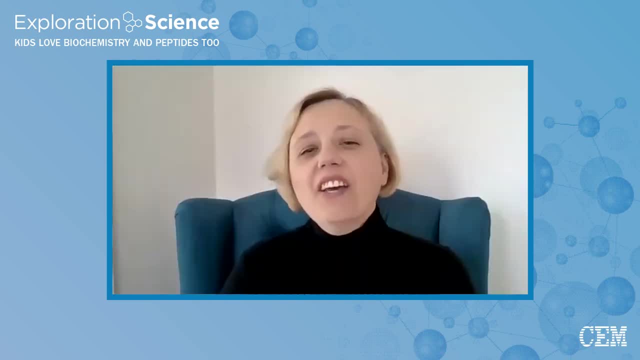 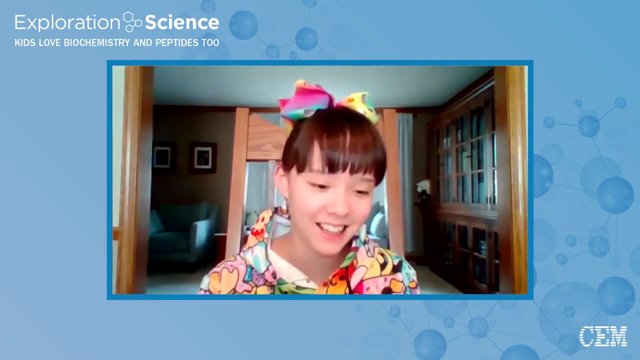 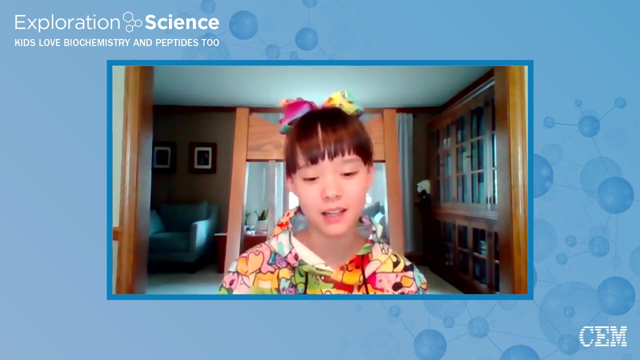 Like one semester ahead or something. Okay, great. So what? um? what so far has been your favorite lesson? Oh, that's really hard to decide. Um, I liked the electrophilic aromatic substitution reactions, but I also really liked the serine protease, because that was the first mechanism I learned. 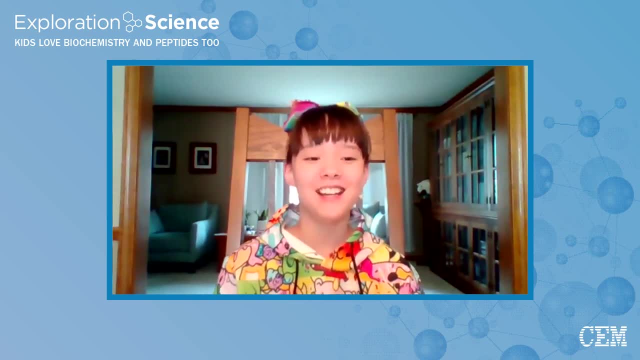 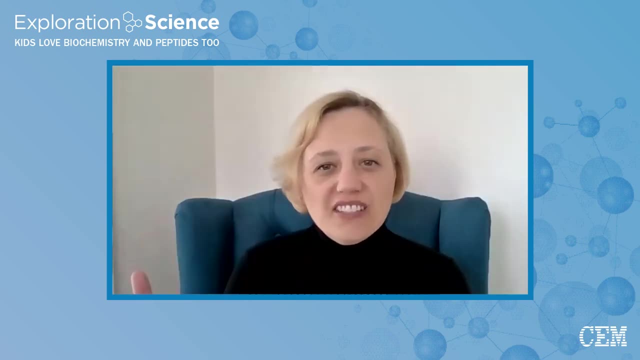 But I also really liked the star chemistry because I'm into astronomy and that type of other stuff. I like to learn, Yeah. So, um, in astronomy, what are your, what constellations do youso? what are you drawn to of the different constellations? 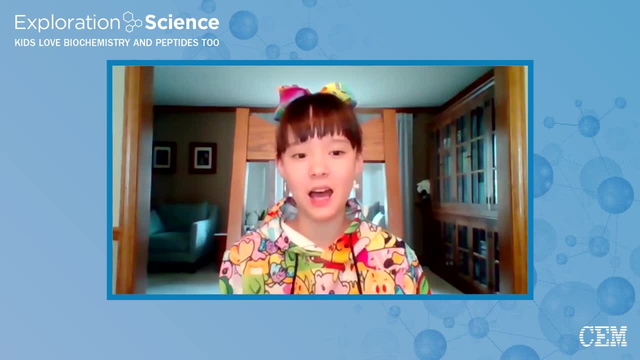 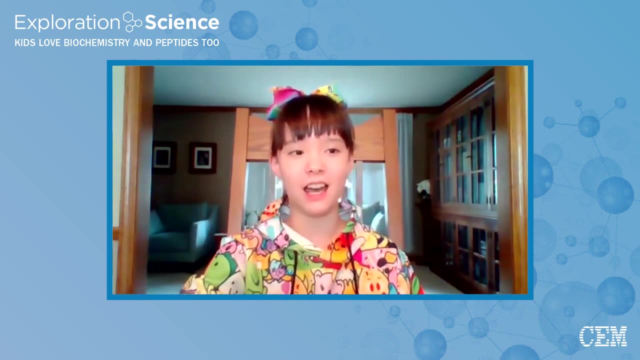 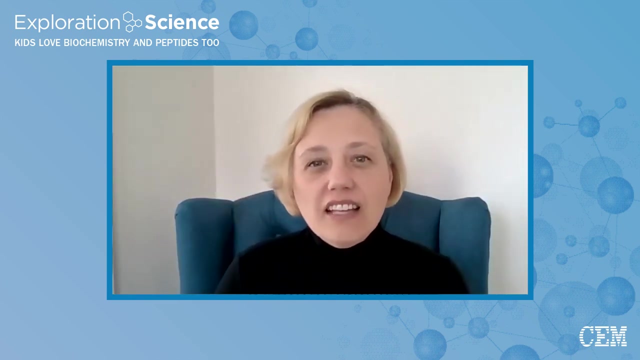 Um, I don't really study constellations. Um, Uh, In astronomy I'm less interested in, like hmmplanetary sciences And I really like cosmology. actually, I know in that star chemistry, um, uh, I guess lesson you guys were talking about the formation of molecules and how molecules came to be about. 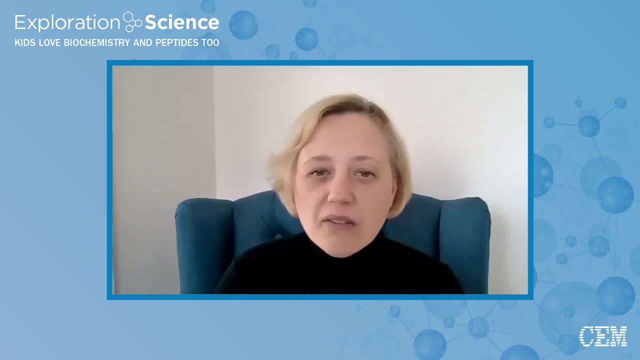 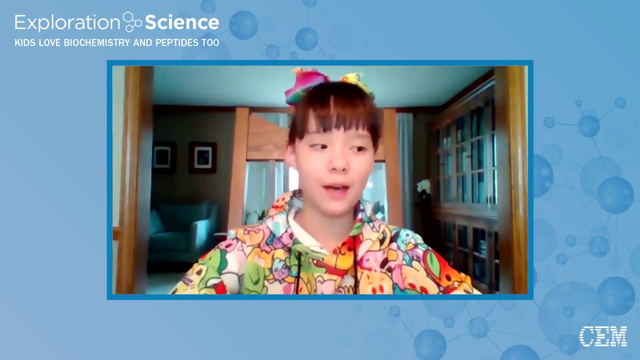 Uh, So, um, yeah, Can you tell me about some of those, those molecules that you learned about? Yeah, so the first thing we learned about was, I think, how helium was created through fusion of hydrogen, which was the easiest part, And then 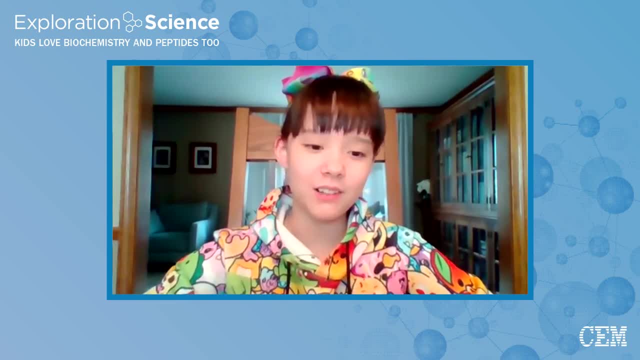 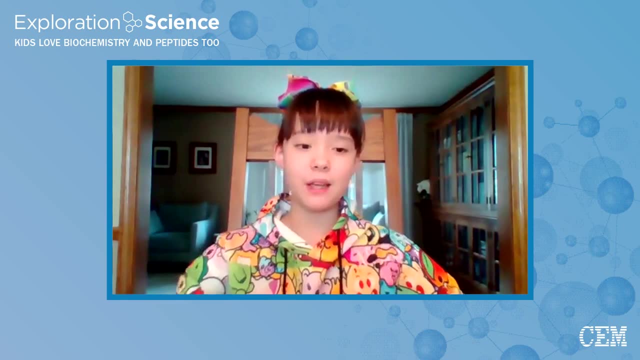 we learned about the triple alpha cycle, which is done in high energy stars and basically fuses three heliums together to make carbon But the stars to be really high energy because of the three body issue you can't. it's really difficult to have three molecules colliding into each other. 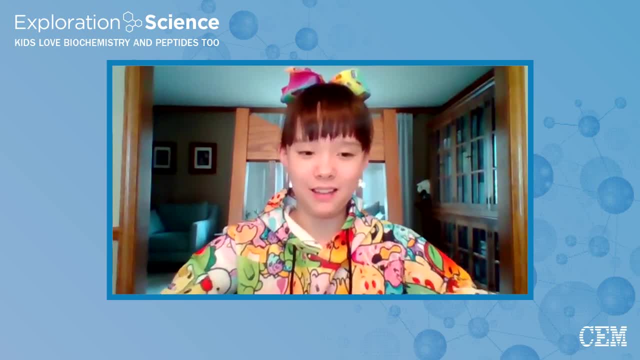 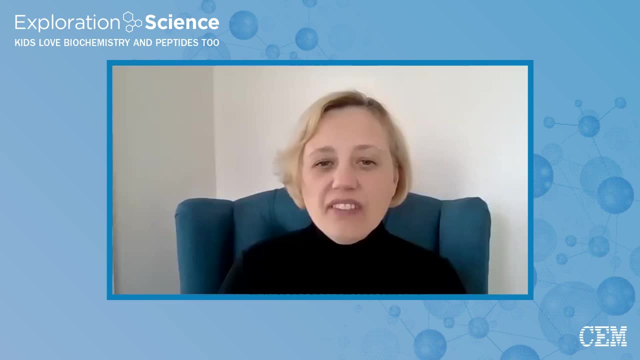 at the same time. So really the only way that could happen is if you had, like a high energy star, And so that was really interesting to learn the different energy levels and how that correlates to the different reactions. Yeah, absolutely Something else that you mentioned. you said you. 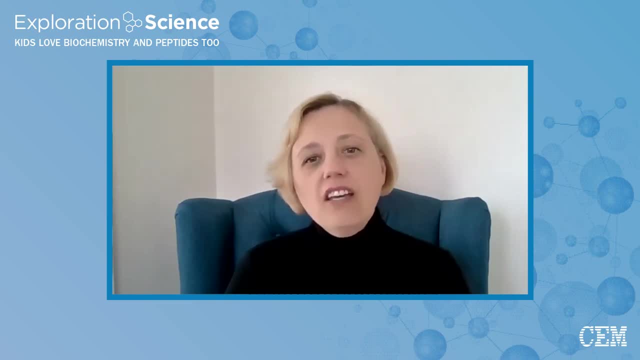 really liked the electrophilic aromatic substitution reactions. Is that some? can you tell me kind of what? what does draw you to that? Are you? do you have like an art background? Do you like drawing Like? do you like the arrow pushing Like? what is it about that? I think aromaticity really draws me. 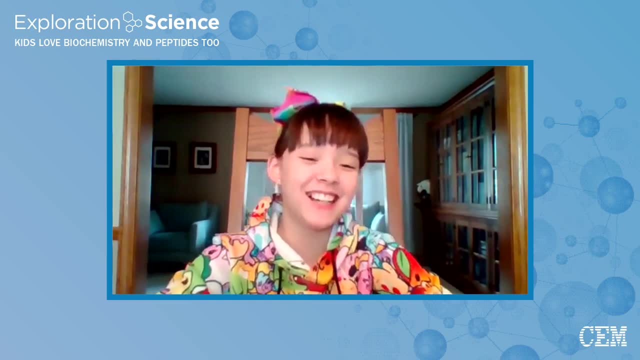 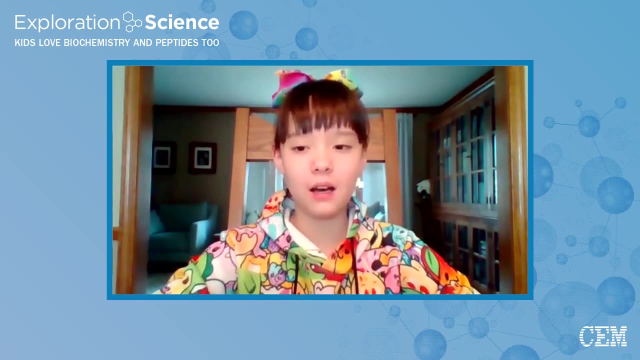 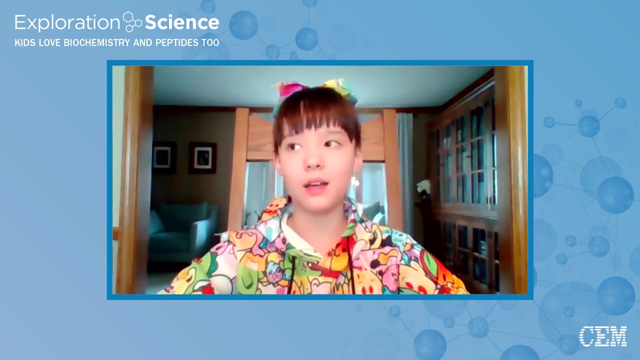 because I also, like I have many interests, but I really like particle physics, And so resonance was really interesting to me because it kind of reminds me of like of how just it's just the oddness of the quantum world, And so resonance kind of reminded me of 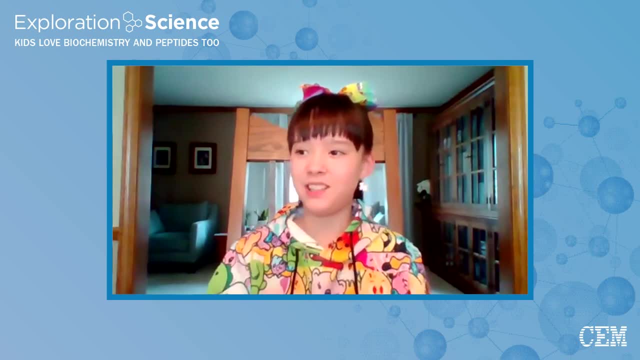 that because, like, how can the electron be here and here? It's never in one place at the same time. So it's kind of like how can the electron be here and here? It's never in one place at the same time. So I liked that. 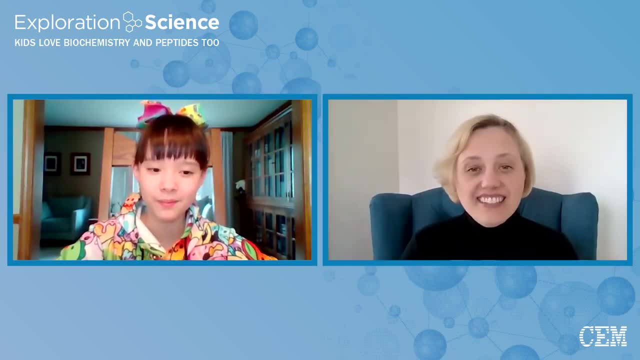 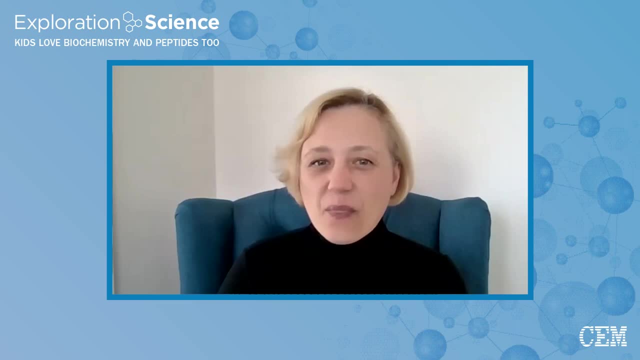 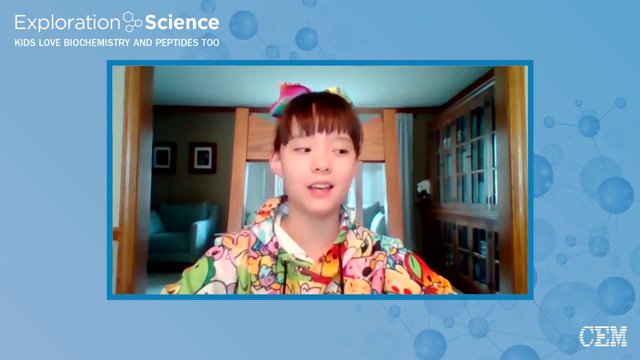 So tell me about some of the other activities that you're involved in. I mean, I do a lot of things. One of my favorite things, of course, is taking Dr Freed's class, but I take a lot of other online classes too. I take math class, an, art class, a- I can't even remember. 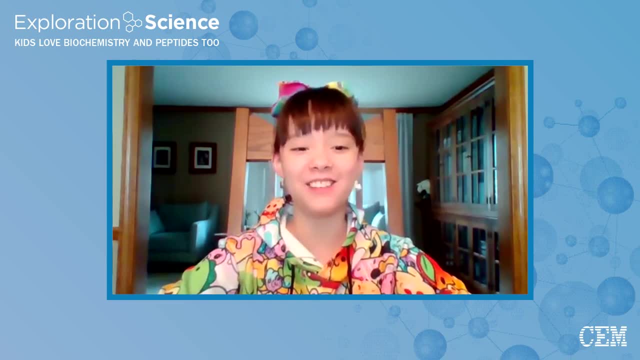 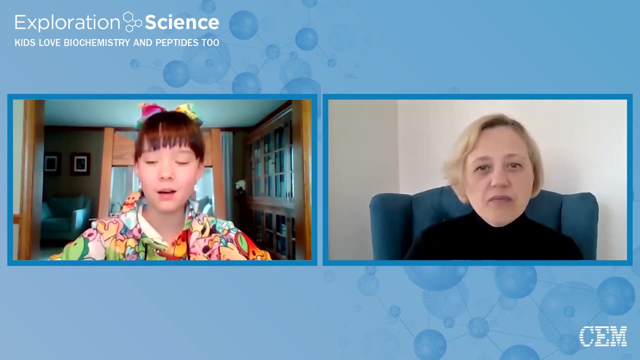 a biology class, a French class, a Korean class, So I basically just take everything. That's amazing. What? what are you learning about in biology? Right now, I think we're on the genetics chapter and dominant and recessive traits. 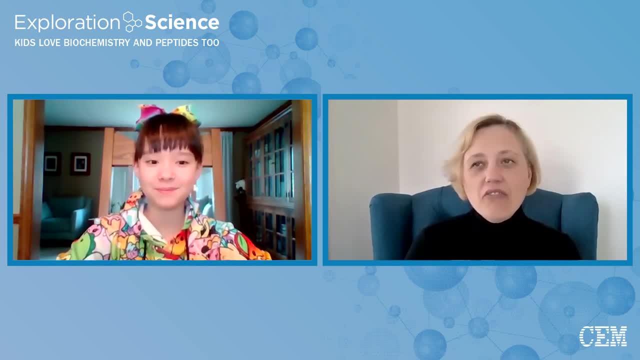 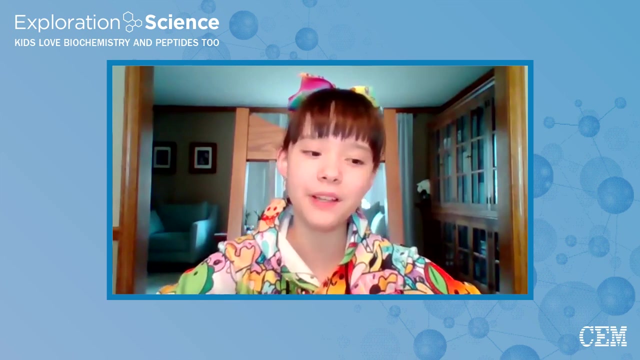 And I like that. It's interesting Very much so. Have you found that taking Dr Freed's class has sort of helped in some of the other areas? as far as making connections between different concepts? Yeah, definitely, Because when I was little I really liked like biology And so 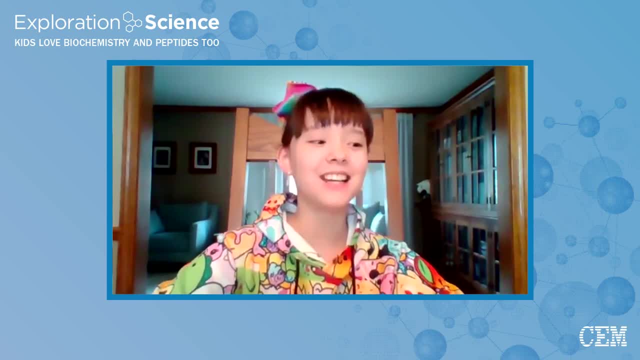 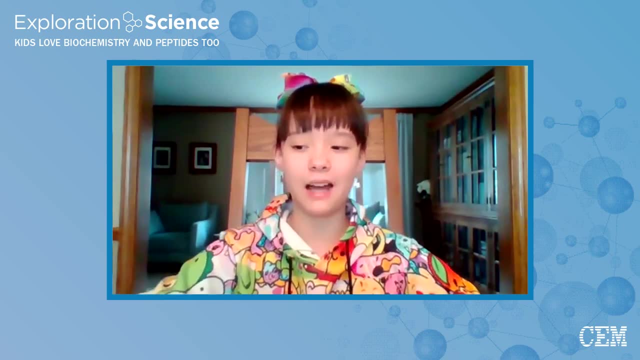 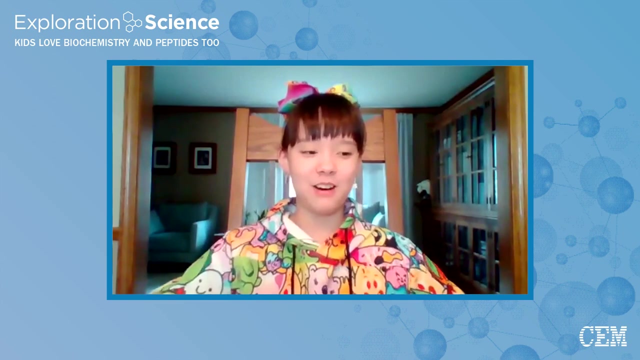 I realized that you need chemistry to learn biology. So that's why I like Dr Freed's class a lot too, because it just chemistry is like a central science. You know it's everything is based on that or leads to that. It's like all roads go to chemistry, Absolutely Yeah. So tell me a little. 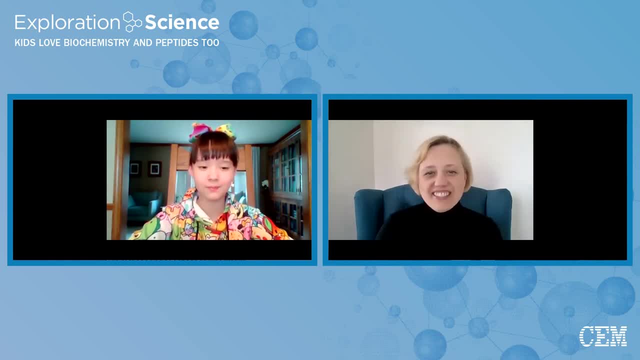 bit about what it's like to learn from Dr Freed. What are some of the things that you like about his class? I really liked that She's not like other teachers I've had in the past that think kids just need to be instructed and they can't really have critical thinking. 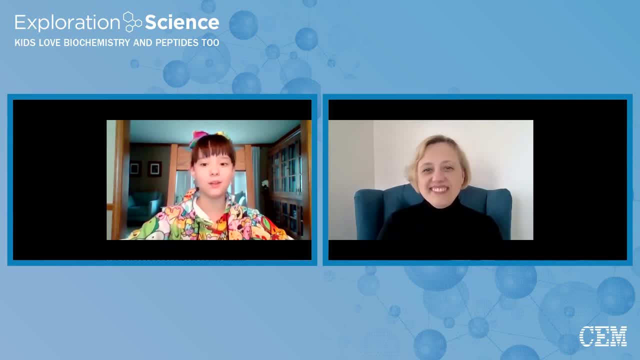 skills. He lets us think for ourselves and use what we know to figure out other things, And he thinks that we can handle difficult concepts. And he lets us ask lots and lots of questions instead of just like saying: you're digressing, we need to get back to the lesson. 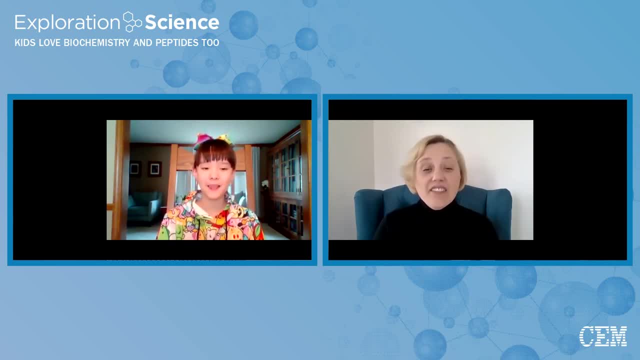 Nice, So he lets you explore other topics as you're learning, And I've seen that in. you know, I've jumped in on a class and watched as he was teaching one concept and questions kind of led through, And I think that was actually a class where he taught aromaticity just on the fly. 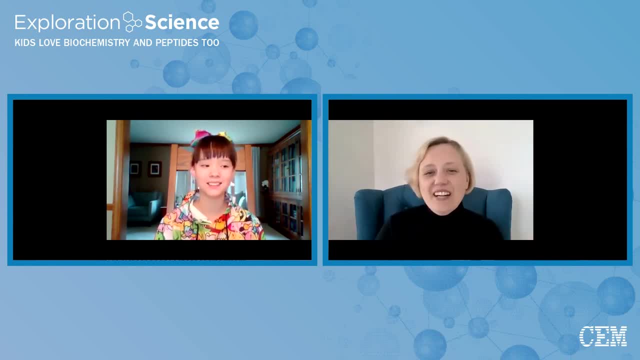 Like it wasn't even planned to do it then. So, yeah, that was really exciting to see. What are some other areas that you're interested in learning about? You know- I know- that, like Dr Freed really encourages guest speakers, you know to have other scientists come in. 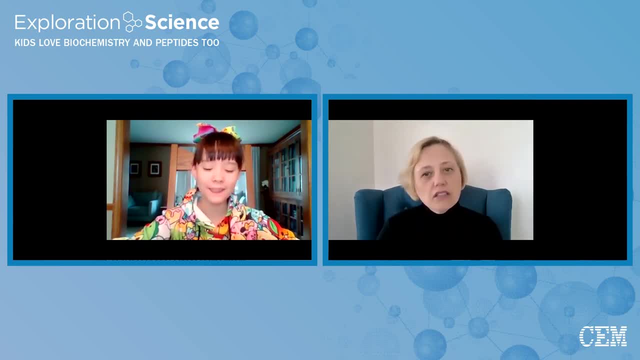 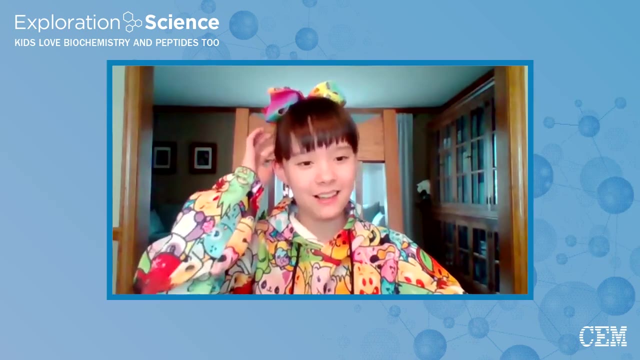 What other areas are you interested? Yeah, I think it would be really fun if he could have someone talk about molecular orbital theory, because a lot of times someone will ask a question and he says that's molecular orbital theory. I would really like to learn more about that. I feel like that would answer a lot of the questions. 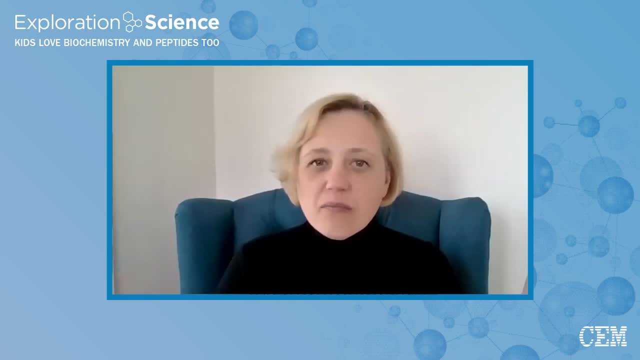 that I have. Have you? I mean, I know you're 10, but you're so you know, I guess, what's the word. You've had so much exposure to so many different things, right, Science, art, language. Have you thought about what you? 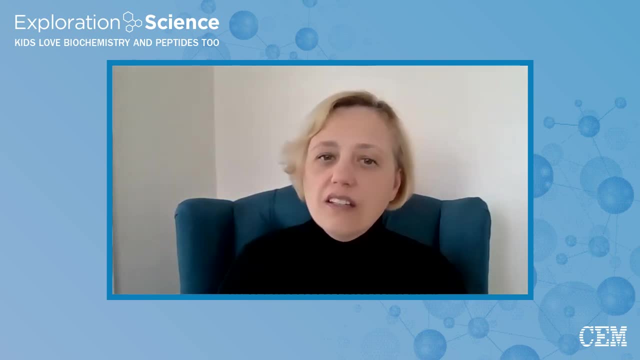 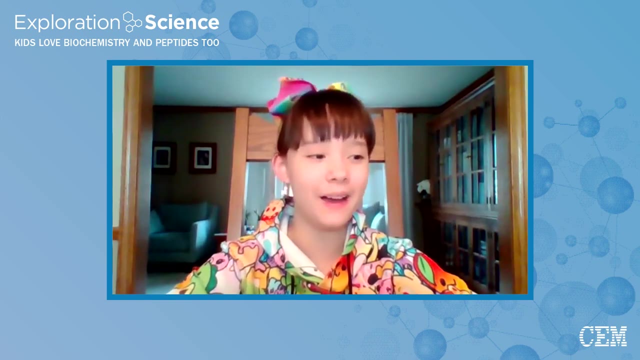 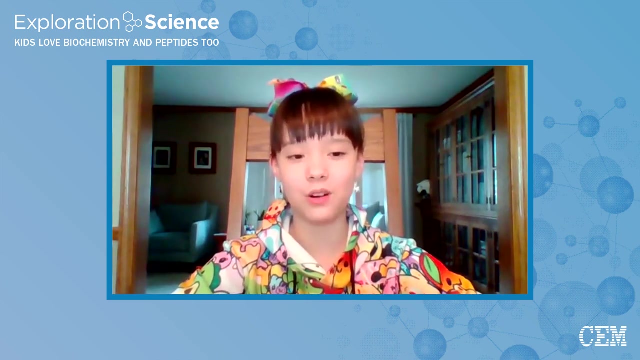 want your career to be, or maybe what direction you might go in. So it's always evolving for me, Like if you asked me five years ago I probably would have said a biologist, but as of now probably a particle physicist or an astronaut, because I like. 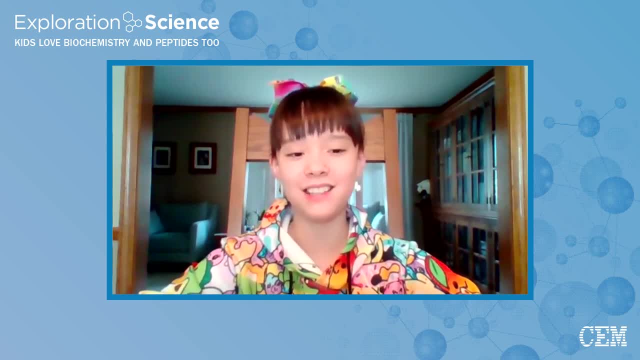 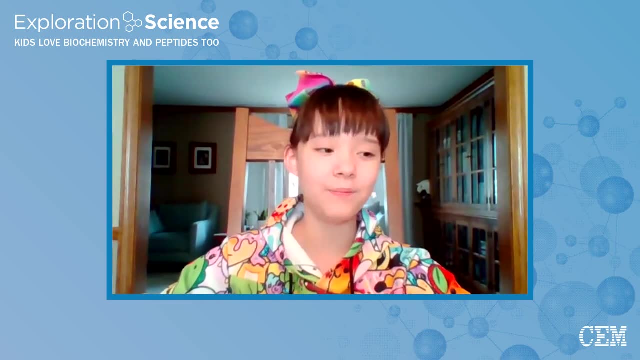 particle physics because it's the most basic of the basicness. So, like all your questions can be answered by quantum physics. And it's just so weird how things work, basically like the opposite of classical mechanics, Like you can't have things move through solid. 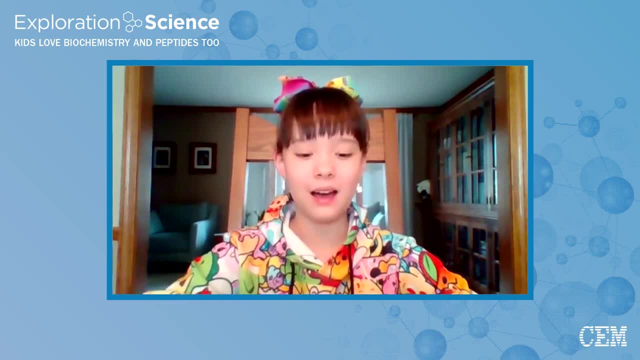 walls, but quantum objects do that all the time, And as an astronaut I really like to just learn new things, and just for the pursuit of knowledge. you know no other reason. So that's why that would be, I think, really interesting career. 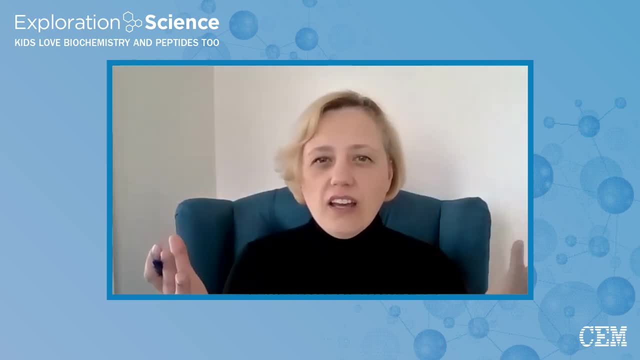 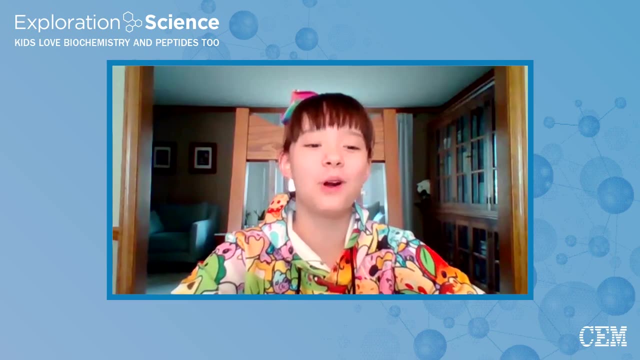 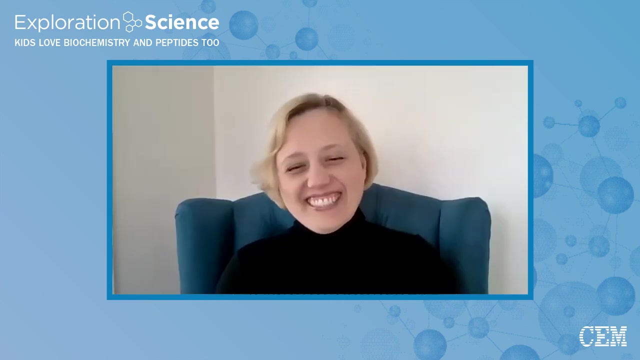 Definitely, Definitely, Yeah. Can't you be an astronaut and be a particle physicist? I don't know? Just both of those jobs take like a lot of work, Okay, So you know, in my dream world, yes, Yes, Okay, I definitely understand that as well. 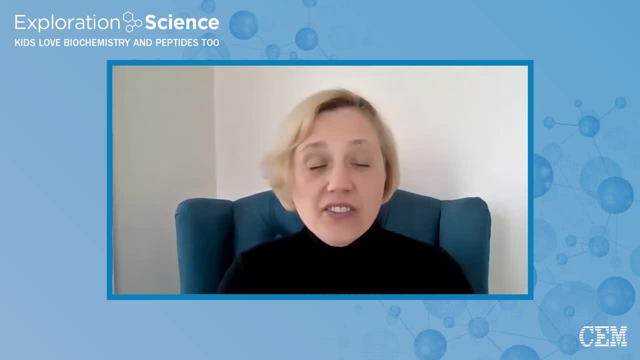 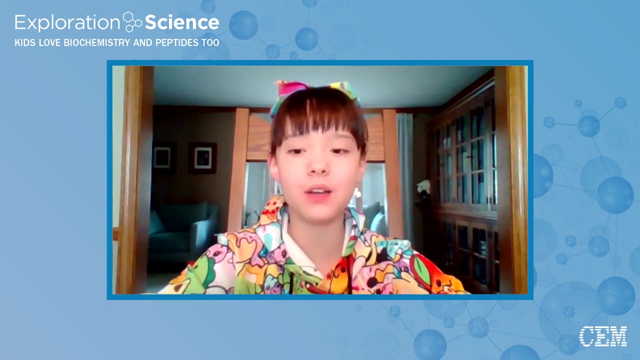 So I know some of your favorite reactions. now I know you said you like searing proteases as well. Do you have a particular molecular class that you're most interested in, Like maybe proteins versus DNA Versus small molecules? Probably something that really talks about how resonance and aromaticity really work, like 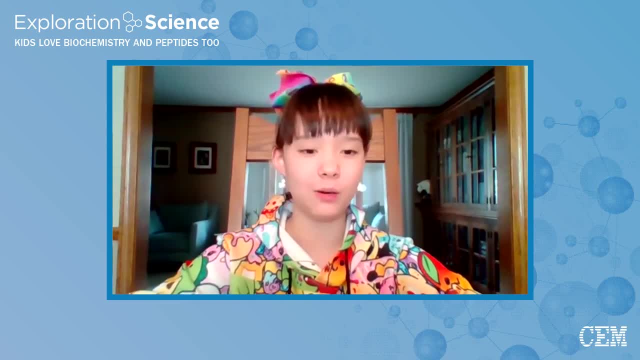 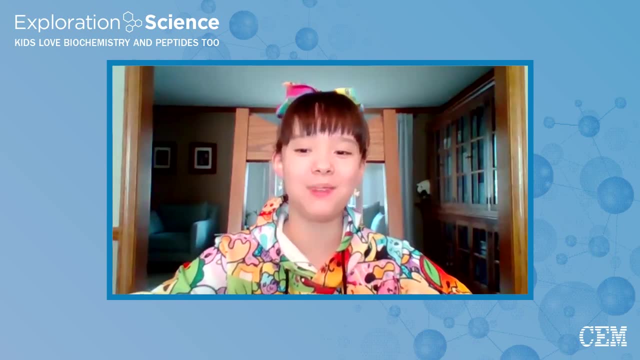 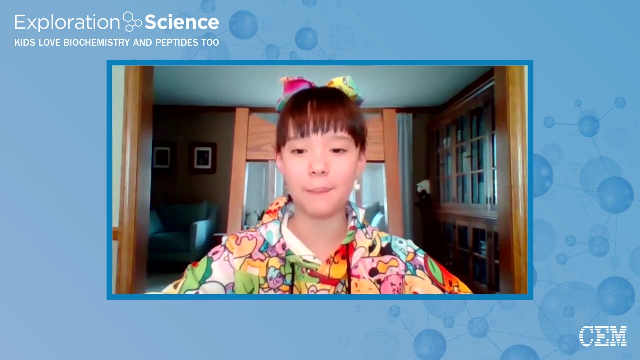 the basic fundamentals of that, which again leads back to molecular orbital theory, as I was saying, Yeah, And also my favorite molecule is nitrobenzene, partly because it's aromatic. So I think that would be a class that I would really like just to really dive deep into that topic. 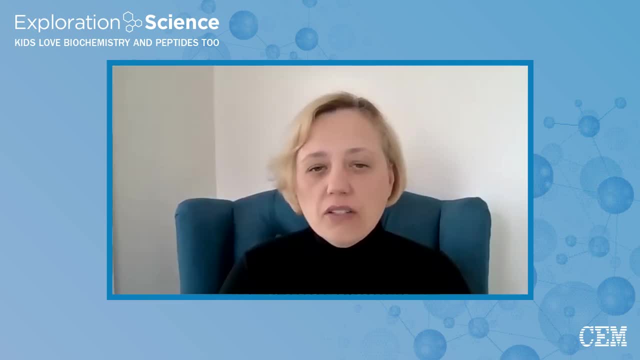 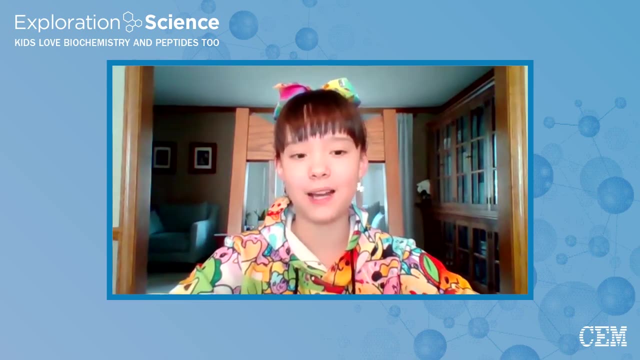 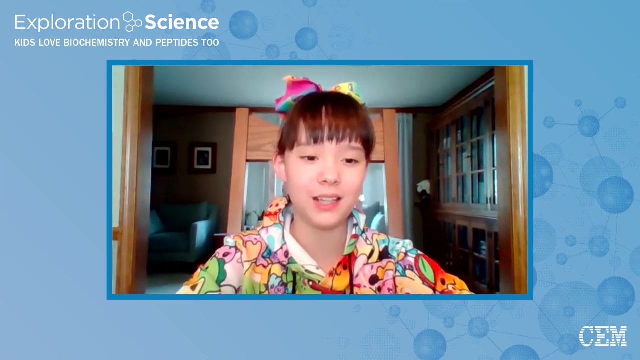 Yeah, What else about Nitrobenzene do you find to be interesting? Well, I think I currently have an attachment to it because that was the first electrophilic aromatic substitution reaction we did And it was just a lot of fun for me following through and drawing and building it and just restoring. 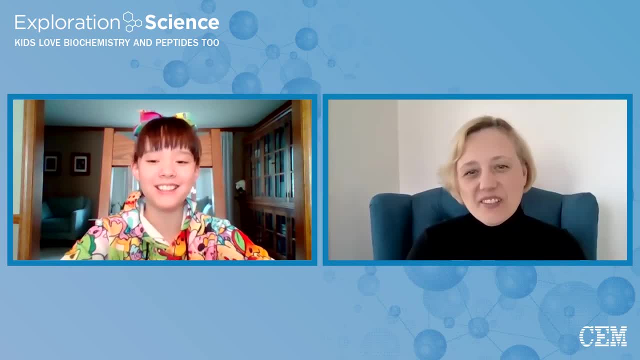 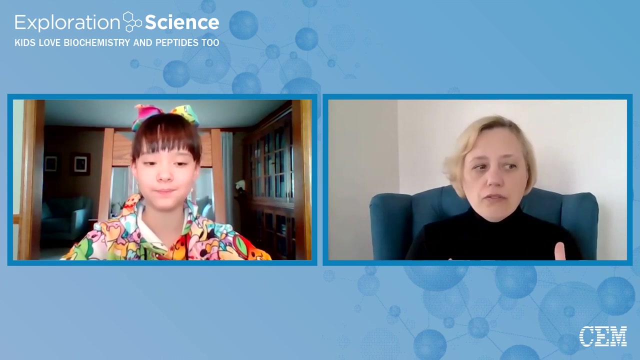 aromaticity and all that. I just it was so fun. So do you on the. you know, I know that you used those models that, the molecular models that Dr Freed has available. Do you and you all also use pymol for like larger biomolecules, right? What do you find as far as platforms? 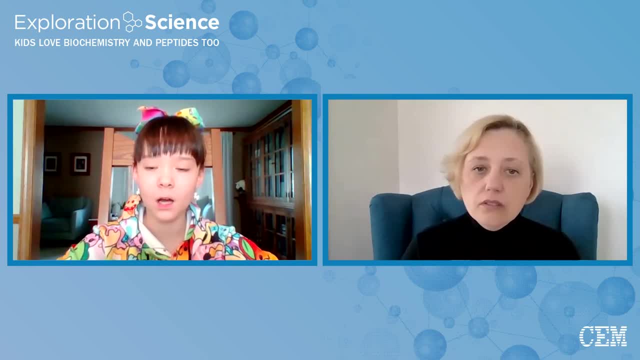 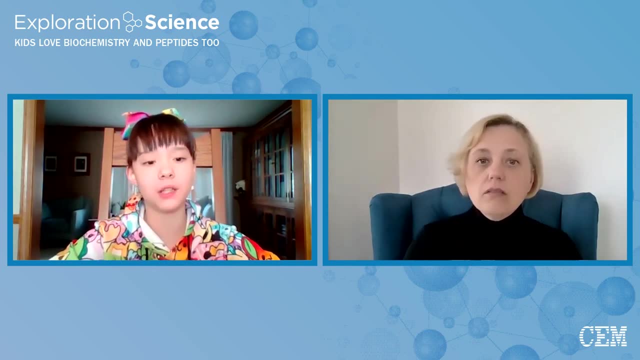 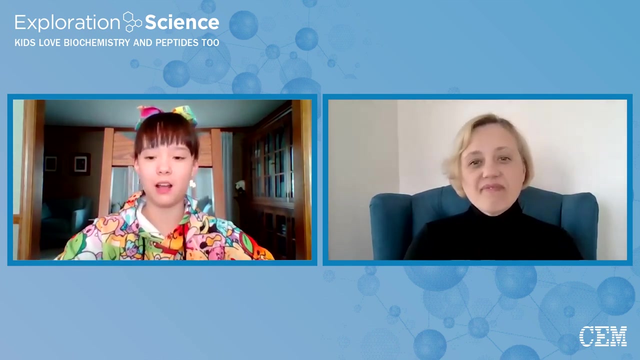 has been the most useful for you. I think the moly mod really helps me to visualize the reactions like restoring aromaticity is something that I couldn't really picture in my brain without the moly mod, So that helped me see how the orbitals- I mean the electrons- would restore themselves. 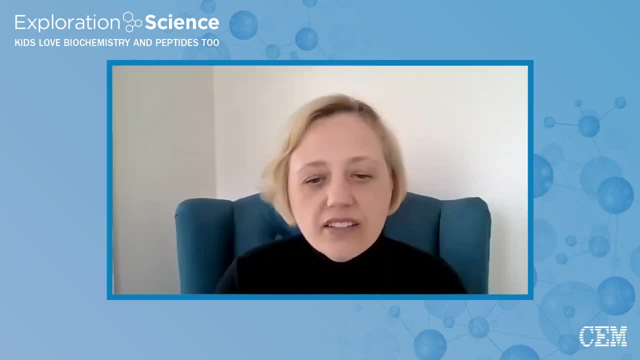 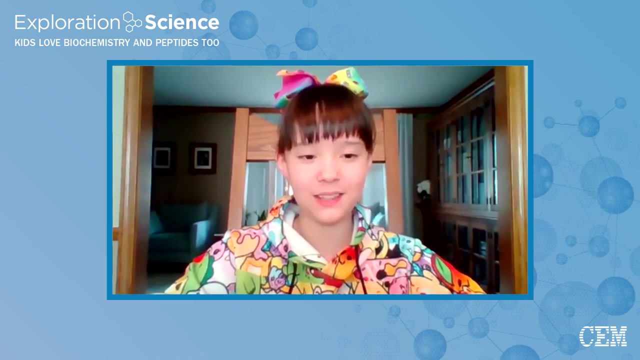 Right. So I think moly mod are really useful. Is there anything else? maybe that I didn't ask you, that you wanted to talk about, about yourself or about what it's like to be in Dr Freed's class? I think that just because you like to study and learn doesn't mean that you can't have a life. 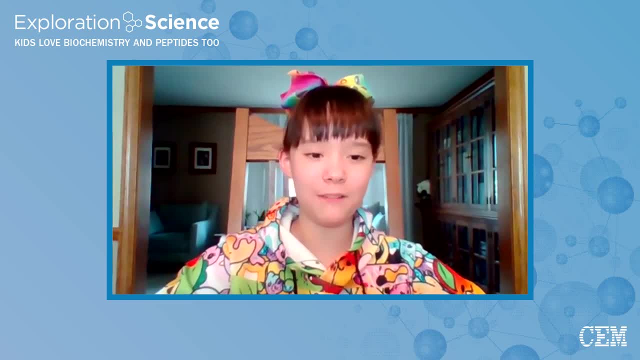 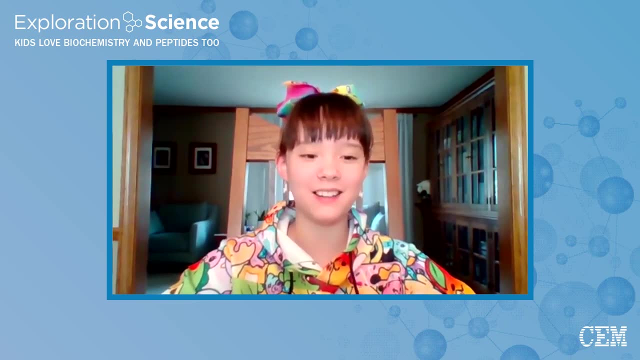 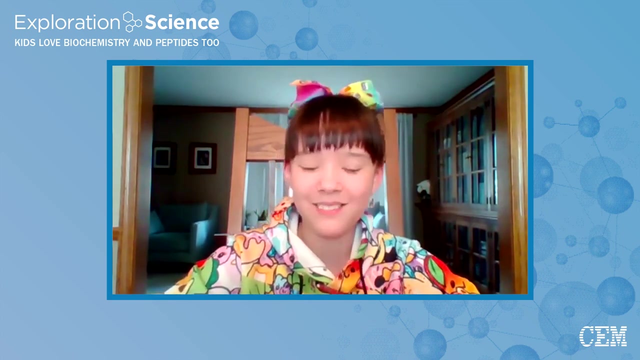 outside of that, Because, like, I do first Lego League with my friends and we have a great team And I do violin and piano and I swim and I play tennis. So I guess, just for anyone listening, just because you like biochemistry, for example, like me, 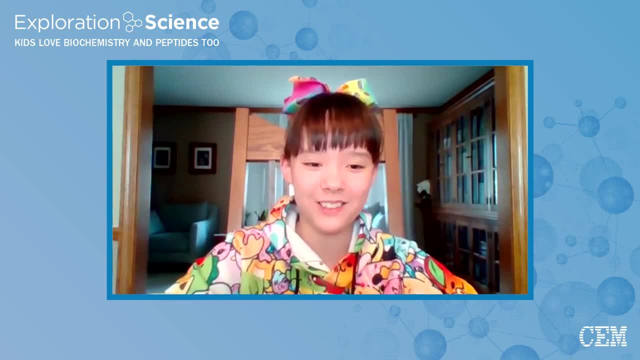 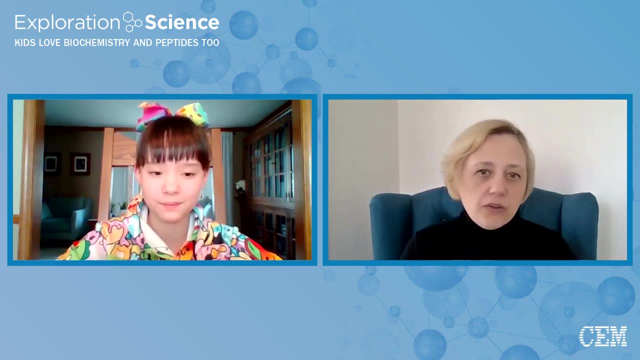 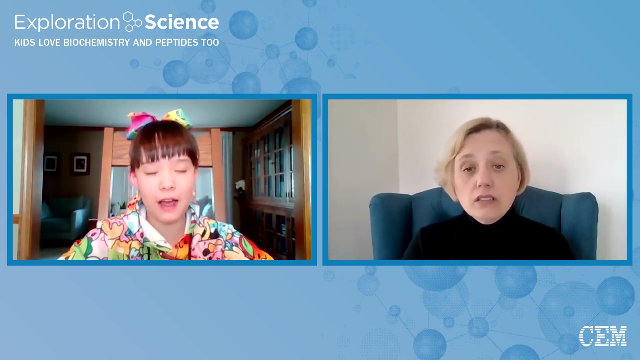 that doesn't mean you can't like anything else. You can have a very varied interest. Yes, absolutely Yeah. you had mentioned even doing art. right, But what sort of art do you make? I do a lot of digital art, like very graphic, sort of like anime and stuff, And I also like to 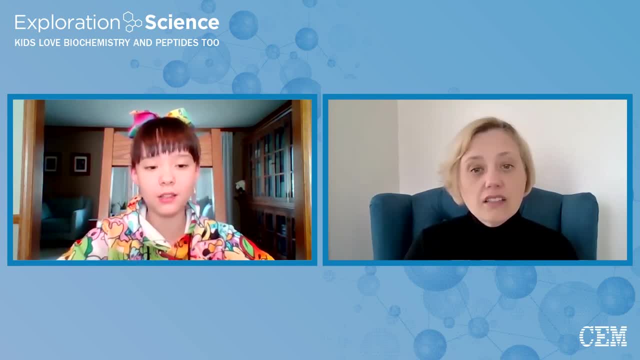 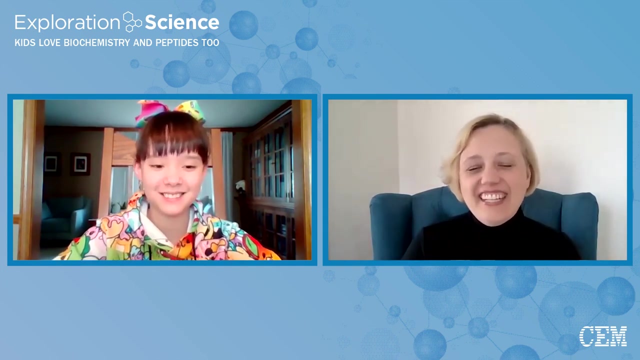 do, uh, just art with pencil and acrylic painting. nice, that's awesome. yeah, i also i love acrylic. by the way, i'm not not very good at it, but i don't care, i still like to do it. i like it for the texture that you can get out of it. yeah, that's a lot of fun. it is um well, um, you know, i really 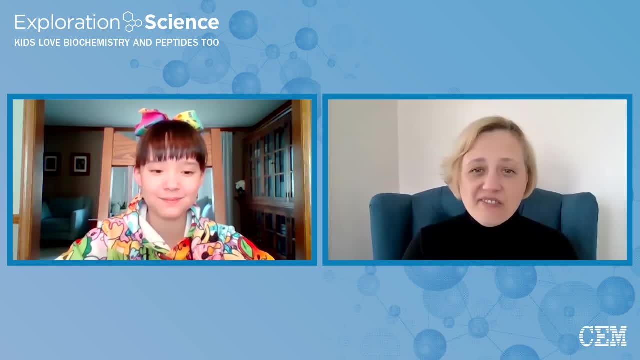 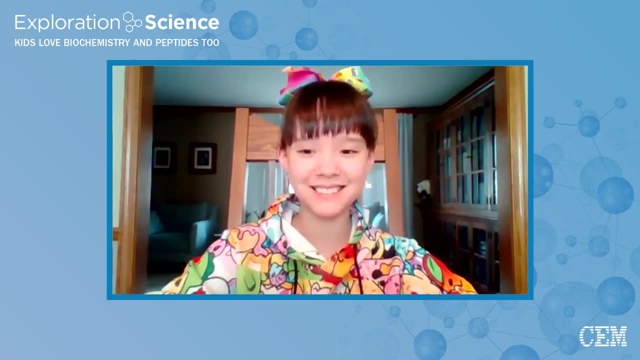 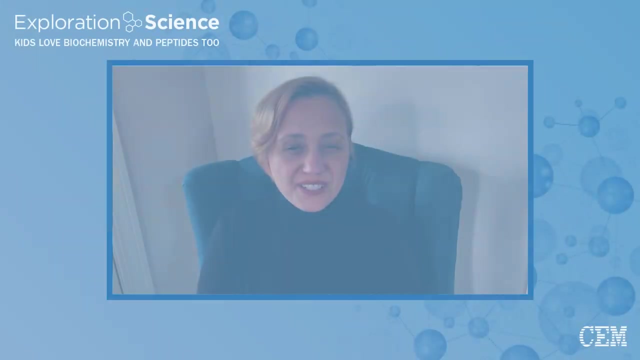 appreciate your time and your answers. they're so very thoughtful and i love again, i love your hoodie, i love your bow. thank you all right, katie. well, thank you so much for your time. i really appreciate it. you're welcome. thank you for tuning in to this episode of exploration science if you enjoyed this.